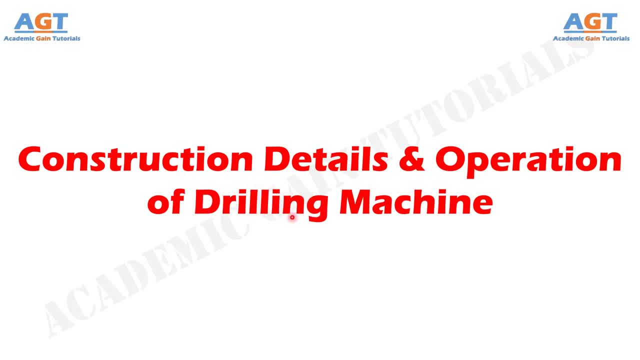 It is one of the most important and versatile machine tools in a workshop. Besides drilling round holes, many other operations can also be performed on the drilling machine, such as counter boring, counter sinking, honing, remming, lapping and sanding. 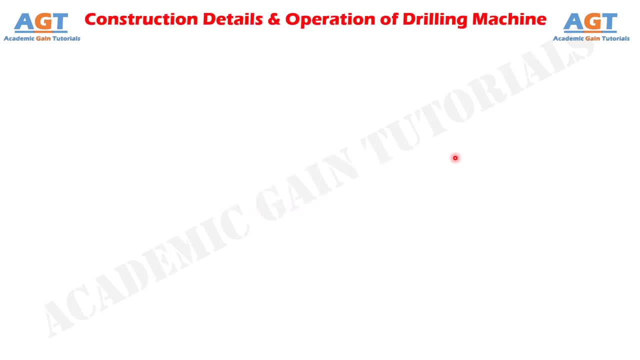 Now let's look at the construction details of a drilling machine and the operation of different parts that together construct a drilling machine. First of all, at the bottom portion is the base of the drilling machine. It carries the entire weight of the machine and transfers the weight to the ground. 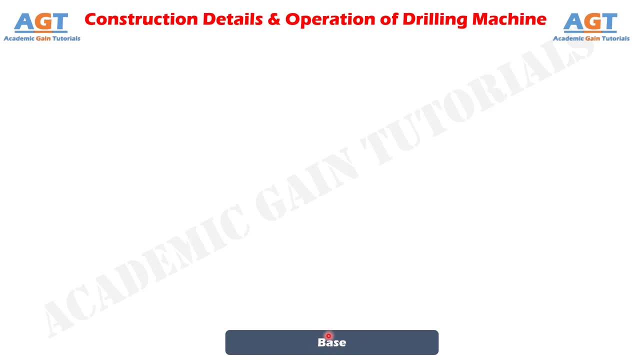 The base of the drilling machine is made of cast iron through the casting process, Since cast iron has a high shock absorbance and wear resistance capacity, so it helps the base to absorb the vibration of the full drilling assembly during work and transfer to the ground. 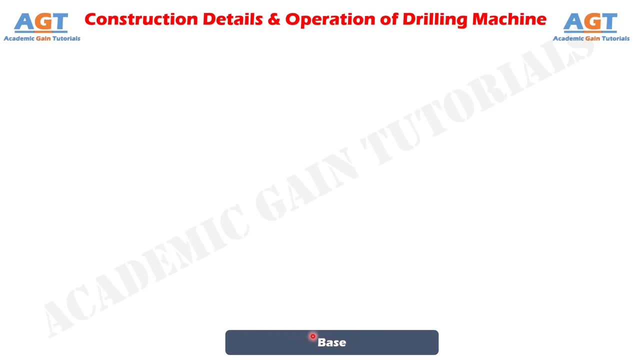 The base is generally bolted with the ground or, in some cases, the base is bolted with the ground. The base is generally bolted with the ground or, in some cases, the base is bolted with the ground. In this case, the base is supported by two or four legs. 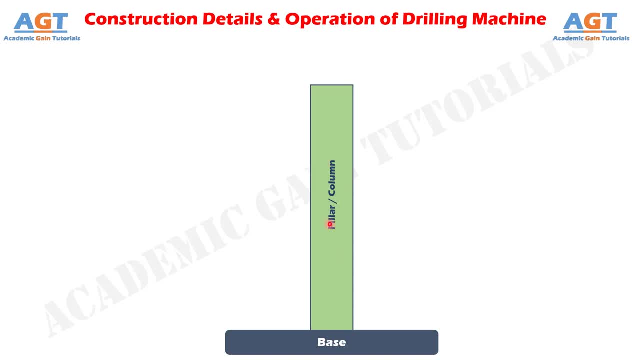 Above the base there is a pillar or column. The pillar is a type of vertical column that usually rests at the center of the bed. The pillar provides support to the motor and the spindle head. This column is also made of cast iron or steel and is very rigid so that it can carry the 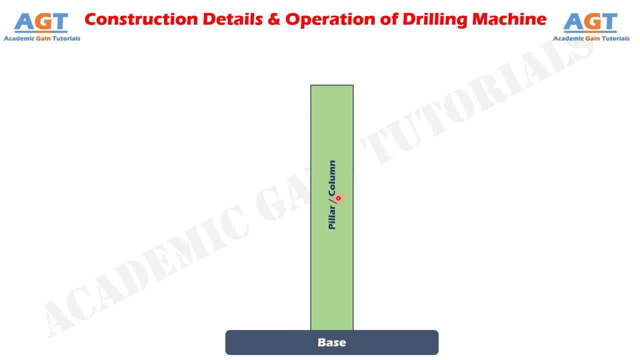 load of the arm, as well as a drill head. After that, mounted on this pillar or column, there is a swivel table. Some may also call it a sliding table. The table is attached to the base. The table is attached to the column and it can be rotated around the column at any position. 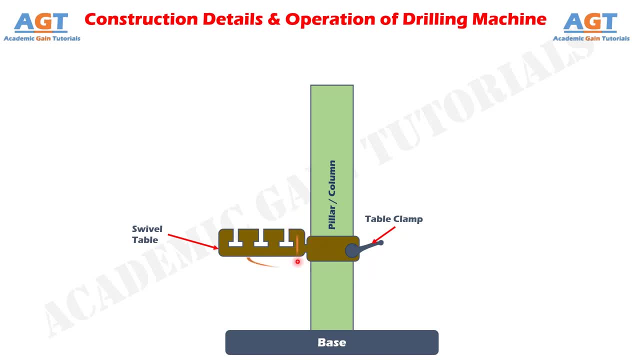 and can have an upward and downward sliding movement along the column. There are T-slots cutted on the swivel table and the workpiece can be mounted on the table using these slots. The swivel table can be adjusted at any position as per requirement. 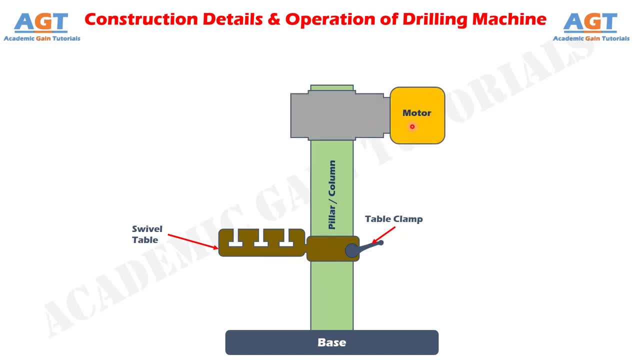 Now up here at the top of the column at one side, we have a motor. Inside this motor there is a shaft which connects the motor to a stepped pulley. So what is a stepped pulley? The stepped pulley usually has three to five grooves with gradually increasing diameter. 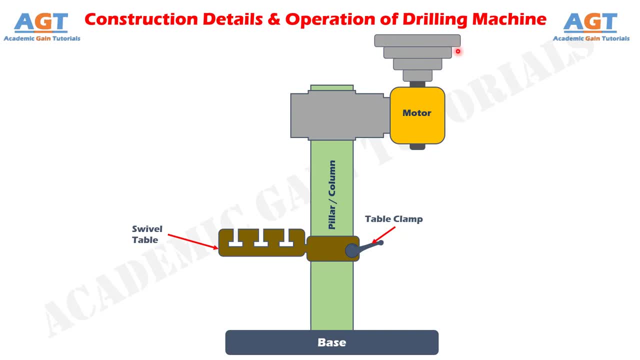 from smaller to larger. Stepped pulleys are used to increase or decrease the speed of the rotation of the motor without having to take the pulley off and replace it with another. So this stepped pulley is connected to the motor through this shaft. 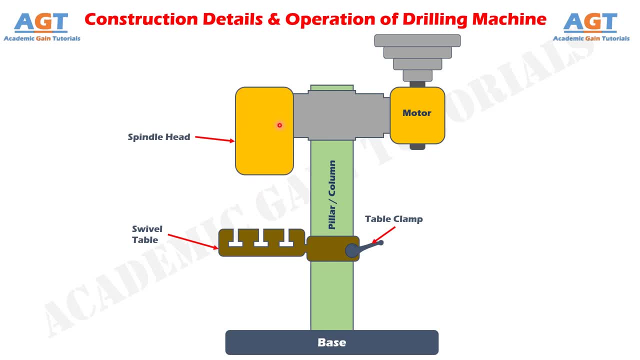 Now, on the other side, we have the spindle arrangement. This is the spindle head or the spindle box, and the spindle is fixed inside this spindle head. It is connected to a stepped pulley above it through a shaft. This stepped pulley is the same as the stepped pulley connected to the motor, but it is mounted. 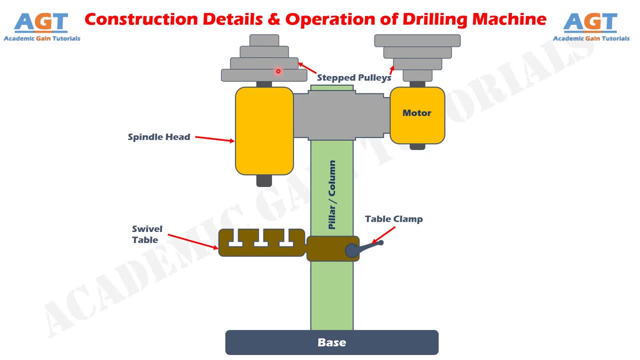 in reverse or opposite direction to the other stepped pulley. For example, if this pulley is mounted facing downwards, then the other pulley will be mounted facing upwards. These two stepped pulleys are used to regulate and maintain the velocity ratio and adjust. 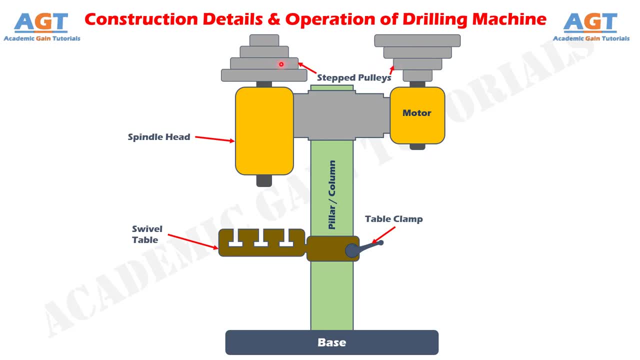 the speed and motion by increasing or decreasing the speed according to requirements during operation. Connected to the bottom of the spindle there is a chuck. The basic function of the chuck is to hold the cutting tool firmly. Usually it holds the drill jig and the drill bit or the cutter is mounted on the drill. 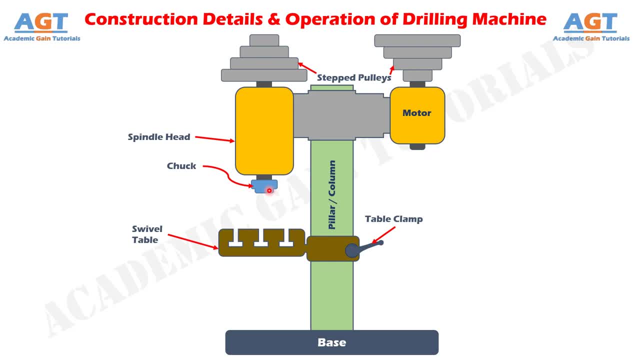 jig, But in some operations the drill bit or the cutting tool can be directly mounted on the chuck without drill jig. This depends on operation requirements, whether to use a drill jig or to mount the cutting tool directly to the chuck. Now a keyhole is also provided to loosen and tighten the chuck tool. 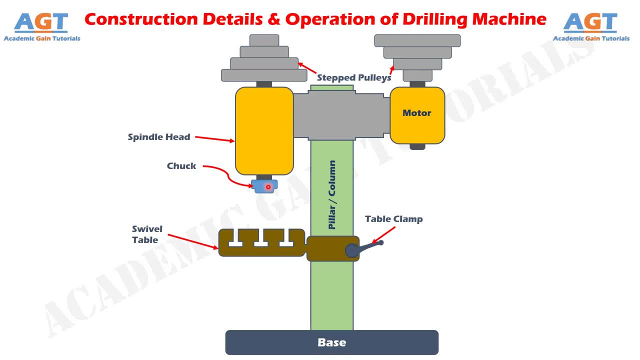 You can check the latter Step 3.. chuck to change the drill jigs. the drill chucks are generally self centering. in a drill machine we use three jaw chuck and it is made of special alloy steel. so the basic function of the chuck is to hold the cutting tool firmly. now the drill. 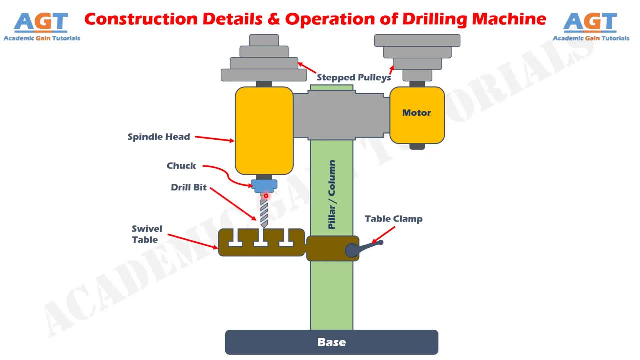 bit is mounted on the chuck. the drill bit is a multi point cutting tool that is used to create a hole in the workpiece. so a drill bit is a major part of this machine and is used to remove the material in the form of holes from the surface of the workpiece. while revolving, there are t-slots cutted on. 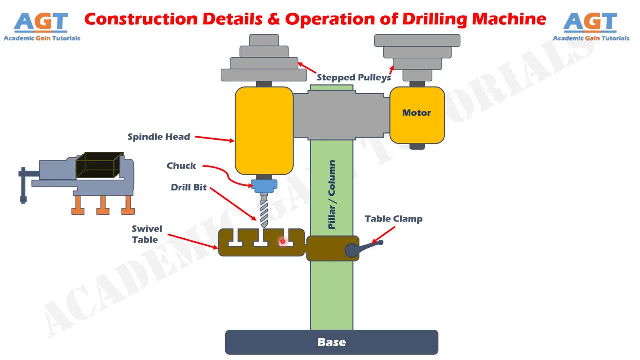 the swivel table over here. using these t-slots, any machine, vice or workpiece holding device can be mounted firmly on the swivel table up over here. there is a drill feed handle or a hand wheel. by rotating hand wheel, the spindle moves up and down in the vertical direction in order to give the necessary amount of 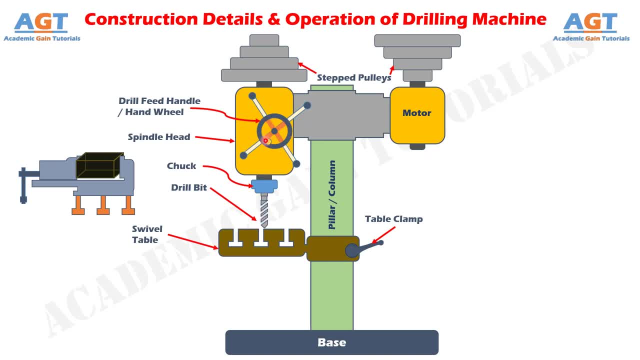 feed to the work. here the rotational motion is converted into linear motion by means of a rack and table pinion mechanism. we will discuss the full working mechanism in a few minutes, but let's finish knowing the construction details first. now a v-belt is placed between the stepped pulleys. we use a v-belt here to connect between the 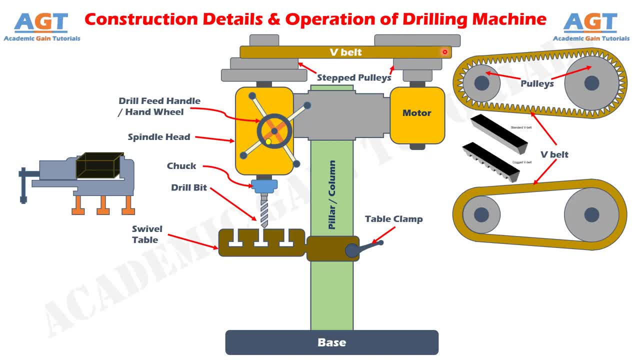 stepped pulleys to drive the power transmission from one pulley to another. so why use v-belt instead of a flat belt? the v-belts have v-shaped grooves cutted on their surface of contact with the pulley. these v-shaped grooves help the 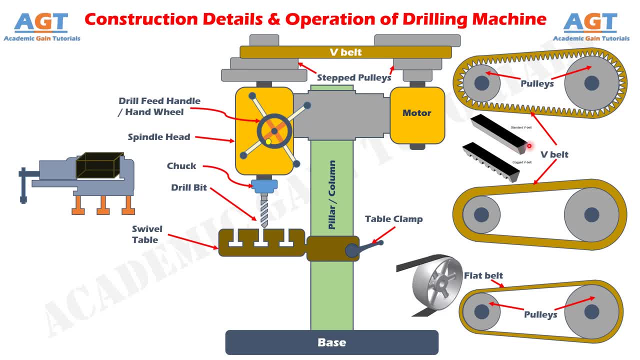 v-belt to sit firmly on the pulley without slipping or sliding away from the pulleys during rotation at high speed, overcoming the sliding or slipping away problem with flat belts. so a v-belt is used here because it is more firm and efficient in transferring motion between the stepped pulleys than using flat belt. so these 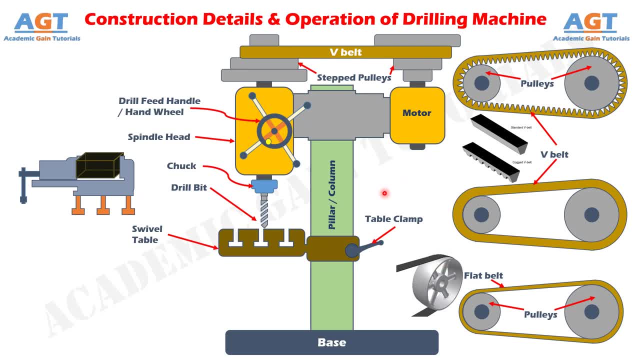 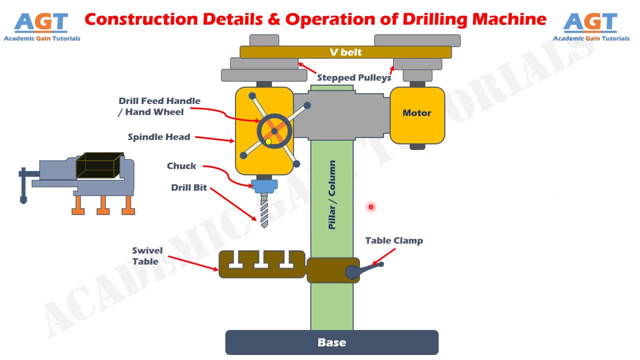 were the main parts that together construct a drilling machine. now let's look into how the parts function for conducting the drilling operation in a drilling machine. first of all, here we have the swivel table that can move upwards and downwards or rotate sideways. along this pillar or column there are t-slots. 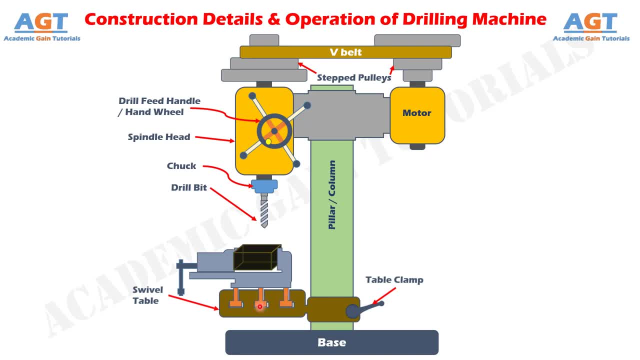 cutted on the surface of this swivel table. the machine vise or work holding device is mounted on the swivel table using these t-slots to lock the machine vise to the table firmly. now the swivel table is adjusted by moving upwards or 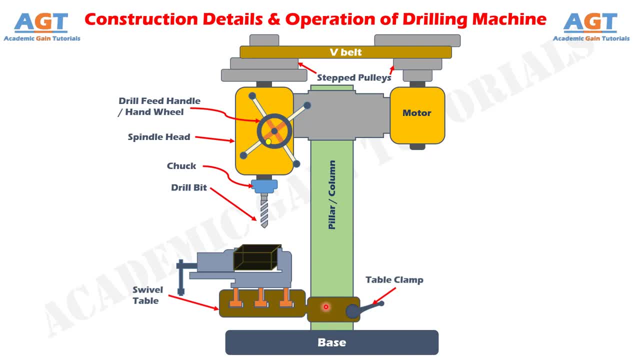 downwards or rotating sideways, along with the machine vise and the workpiece mounted on it. when the workpiece has reached the proper working height or position, the swivel table is locked at that position using this locking lever. now we turn on the switch of the motor and the motor. 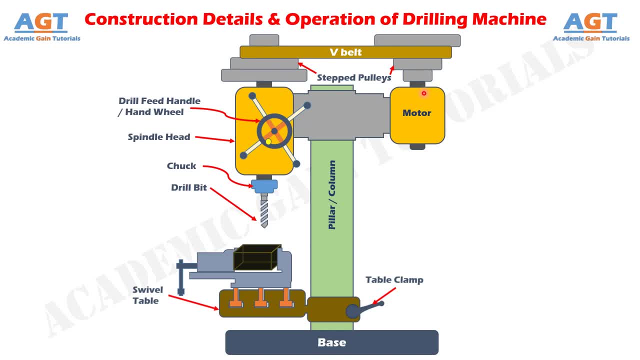 starts rotating, the shaft connected to the motor also starts rotating along with the motor. this stepped pulley is connected to the shaft again. the other stepped pulley is also connected to the stepped pulley through this v-belt. so when the motor rotates the shaft, the shaft in turn rotates the stepped pulley. 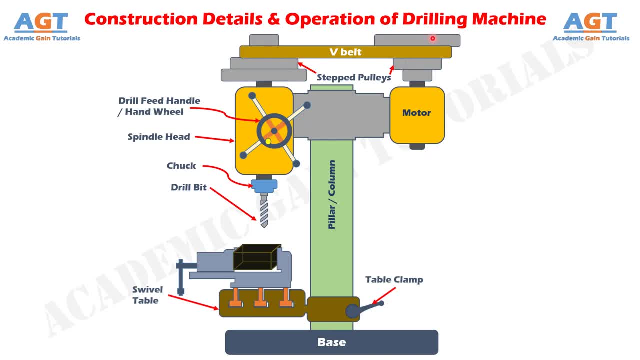 connected to it. when the stepped pulley starts rotating, it in turns rotates the V-belt attached to it. The rotation of the V-belt in turn rotates the other stepped pulley connected to it. Now this stepped pulley is connected to the spindle.